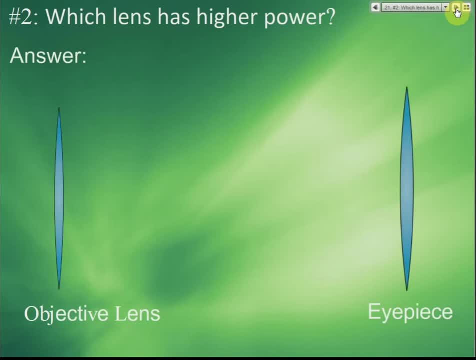 things that you need to know is, among these two lenses- we have objective lens and eyepiece. okay, so they will ask you which lens has higher power. okay, is a favorite question, so in exam, which one has higher power? well, or okay, oh, they ask, they may. 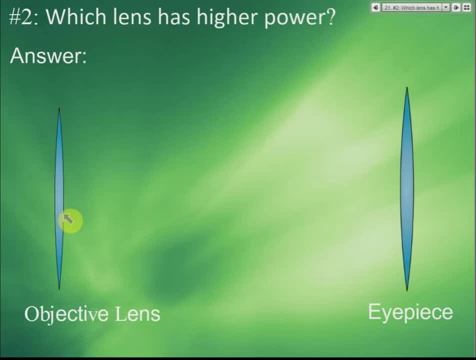 ask you which one has a shorter focus length, or which one is a thicker or whatever. okay, so which one has higher power? the objective lens or the eyepiece? which one has higher power? the answer is the eyepiece. this one has higher power. okay, this one. we try to make it as. 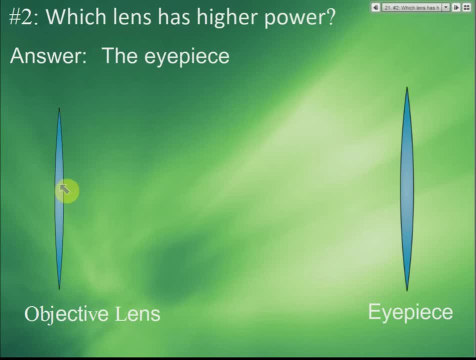 uh, the power as low as possible. so we try to make this as the power as low as possible and to make this eyepiece at the power as high as possible. i will explain to you why later. for telescope, astronomical telescope eyepiece has higher power. objective lens has lower power. 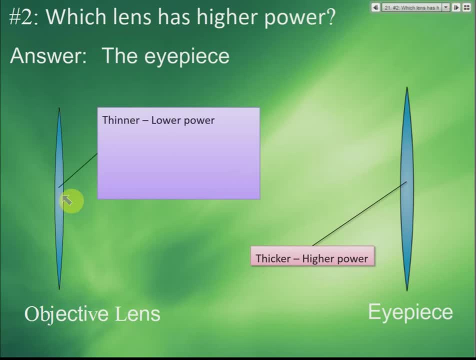 so this is thicker has higher power, this is thinner has lower power. uh, why? okay? why? because because, for telescope, the lower the power of the objective length, the greater the magnification of the image. the larger the magnification of the image means that you will get a bigger image. 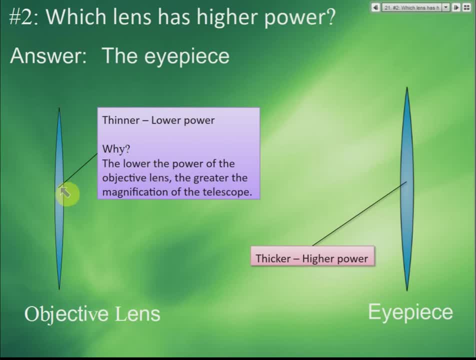 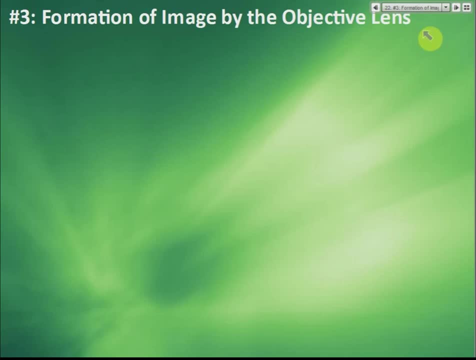 bigger image. lower power, bigger image. so that's the reason. that's the reasons we want to have a smaller power. lower power. for the objective lens: okay. formations of image by the objective lens: so we have objective lens here. astronomical telescope: okay is for us to see something which is 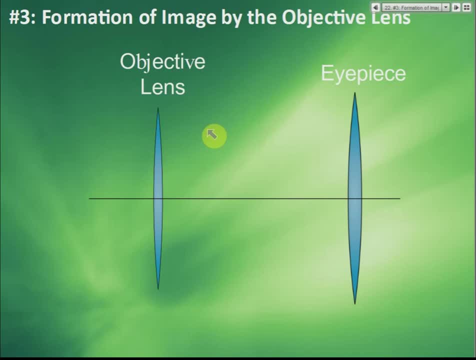 practically so could be f if we were to compare the, how big the intensity of the SE controlled, low, less, and then we would the at the principal focus of the lens. parallel lights, they will focus at the principal focus, so then they will form the image here. so that is the formations of image by the objective lens. 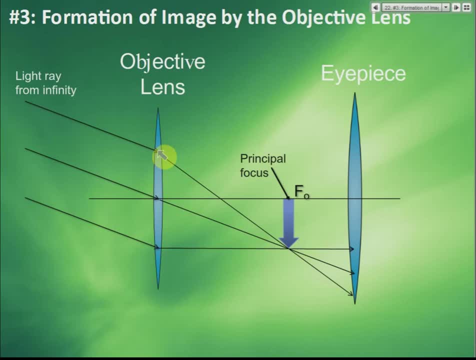 in exam they may ask you to draw the ray diagram. okay, so you need to know astronomical telescope. the light ray is from infinity. so the light ray that you draw is parallel, okay, parallel, not necessarily. it must be parallel with the principal axis. okay, so we can draw three parallel. 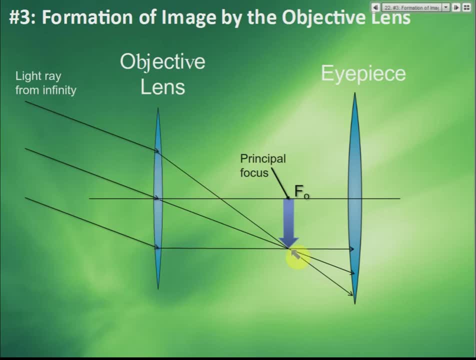 ray and then so this ray, it focus at the principal focus, focus at the principal focus here. so that is the image for the objective lens and the image of the objective lens is used as the object for the eyepiece. this is the image of the objective lens and this is used as the object of the eyepiece. 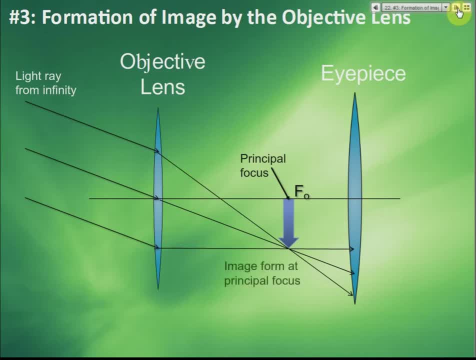 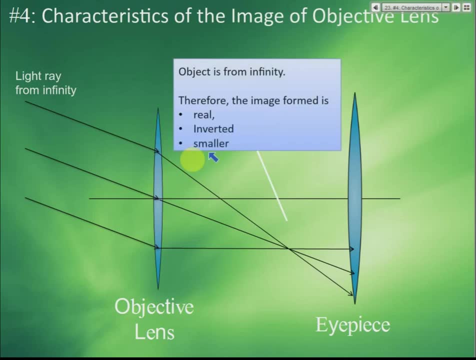 object of the eyepiece, so the light ray reach here. okay, so image form at the principal focus: wake up. okay, so the object is from infinity. so the image form is real inverted and smaller object which is more more than 2f, it's located more than 2f, it will be real inverted and 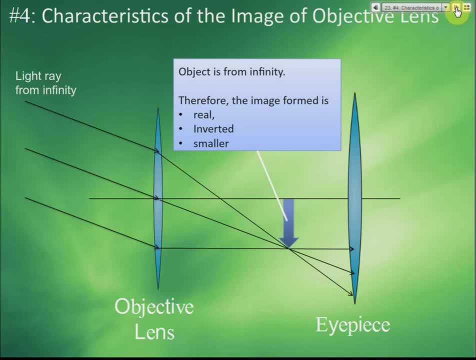 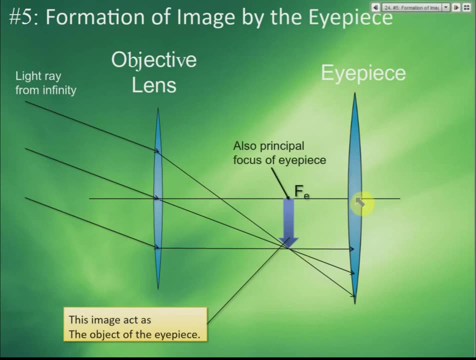 smaller, very inverted and smaller. so this image will act as object of the eyepiece, replace the eyepiece. okay, so that this is the principal focus of the ips. so this is a prince. this point is the principal focus of the objective lens. okay, it's also, uh, purposely placed that, so that is also the principal focus of the ips. 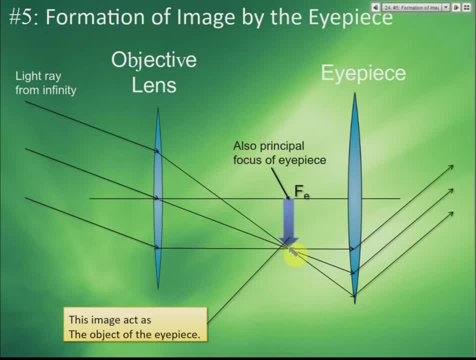 and uh, since this is the principal focus, okay, so the light ray come from the principal focus will be reflected parallel. okay, it will be reflected parallel. okay, all the light rays parallel. so, uh, we, we purposely put it- place the the lens here. so that is, this is the principal. 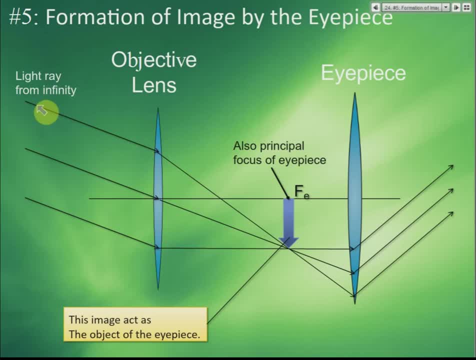 focus so that we can get a parallel light, because the light come from the object is parallel, so here we also purposely put the light ray parallel. okay to do this is that we make this the principal focus of the ips. it's the principal focus of the objective lane, is also the principal focus of the. 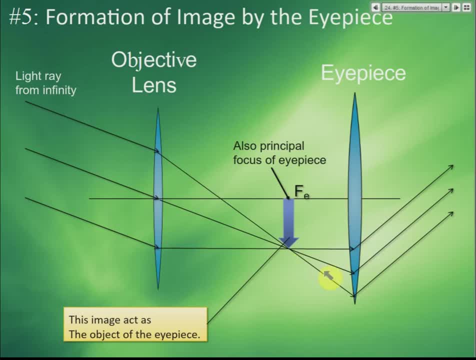 ips. so when you draw a ray diagram you must learn how to draw a diagram. okay, so the ray uh focus on the principal focus and then so after that you reflected parallel, parallel uh, then we extend all these parallel lines to the back and answer then the image form at the back here. okay, 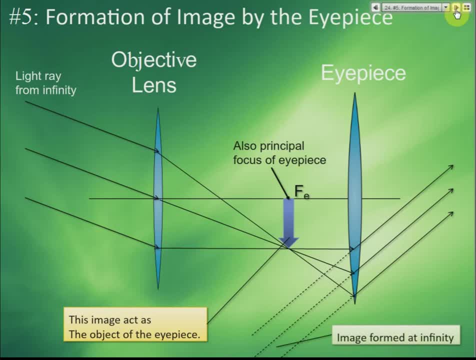 the image form around here. so the image form at infinity, uh, infinity not necessarily must be far, very, very far away. okay, infinity it can be. uh, sometimes it can be, uh, 10 meter away. 20 meter away is considered infinity. okay, yep, but for telescope you can see that the object is very, very far away. 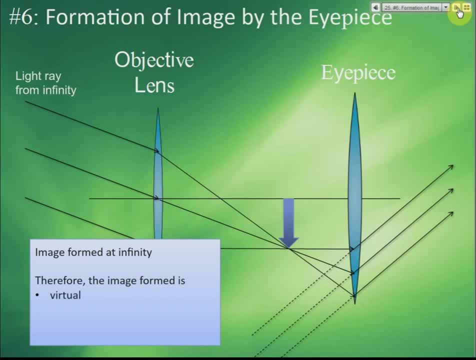 so the object form at infinity, the, the, the image is virtual, inverted and magnify because this one is located at the principal focus. okay, so it's virtual magnify, but then why is inverted? because before this we learned that if we put the object at the principal focus, the image will be virtual. 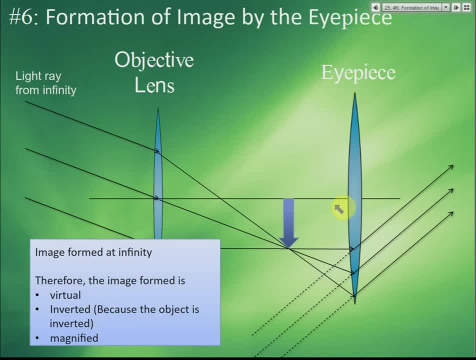 upright and magnify. virtual upright and magnify, but why? why? for this one, then, is the virtual inverted and magnified. okay, that is because the object is inverted. you see, initially the object is upright here, okay, but this is the object for the objective lens, this is the object for the objective lens, and then so you form an image which is inverted, and this: 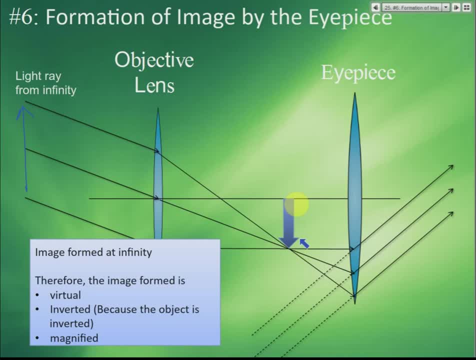 is the object for the eyepiece, and for the eyepiece, the object is inverted. okay. for the eyepiece, the object is inverted. so therefore, uh, the image that you see is also inverted, okay. so, for example, if you see, you use this telescope to see moon, so the moon looks something like this: 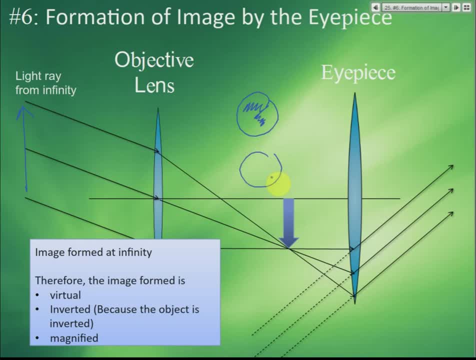 okay, but in the telescope you will see the moon. look something like this: this is the moon, but this is what you see. it's inverted. you will find that the image is inverted. so that is for normal astronomical telescope. okay, so you shouldn't use a normal astronomical? 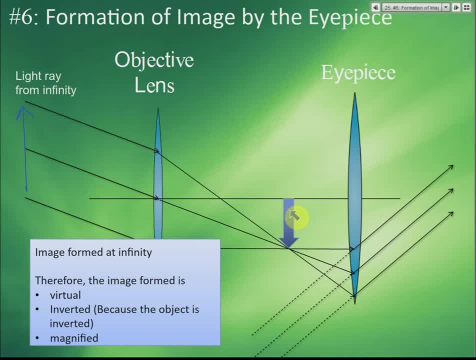 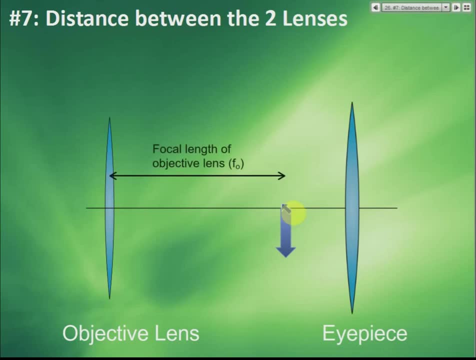 telescope, for sightseeing or what? okay, because the image form is inverted. distance between two lenses? so, uh, you will see there, the policeman will be 따 grasses one, okay, but no, no, you need to. you need to put a very small distance between objects. this is nothing to do with focal length. 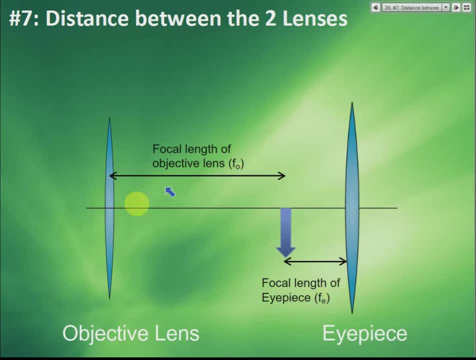 only focal angle focus on the piece of lens you're going to focus on. the straight crossる focal length is the FO focal length of the lens. isn't that spoke about the the focal length of the object discussion project also that this is principle focus on the objective stuff. so therefore, from here to here is the focal length FOF. focal length Oh means object, uh, focal of the objective links and is also the principal focus of the eyepiece. so the distance between this object of the eyepiece is also the focal units focal range. so FO is the focal of the eyepiece to the eyepiece. if E European still theMR has a focal length like this, there's a focal length of the eyepiece. so therefore the distance between this two lenses from here to here is FO.